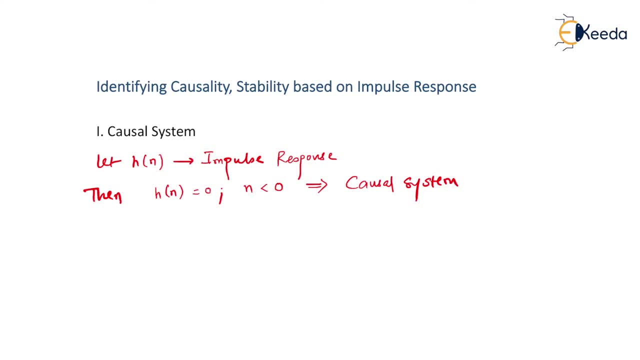 then the resulting system is called as non-causal system. So I would just write else: system is non-causal. So we have written: h of n equal to zero of n is less than zero. nice little, they are very contained components and are totally equal to zero. 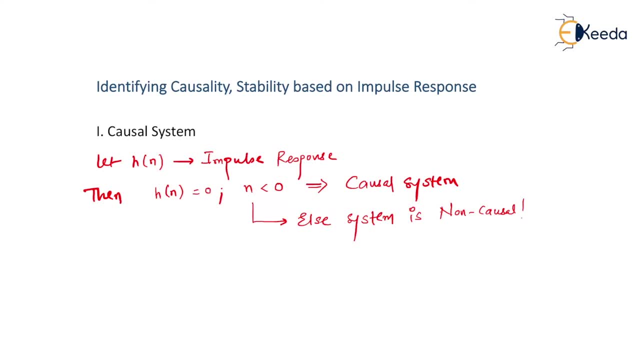 Let us look at another example that we can specifically among the other two types of inputs, where p of i only standards to be causal. So when we actually studied classification of system, where we have understood the dependency of output on input and depending upon that we used to identify whether the system is causal or non-causal. So let me remind you, if the system 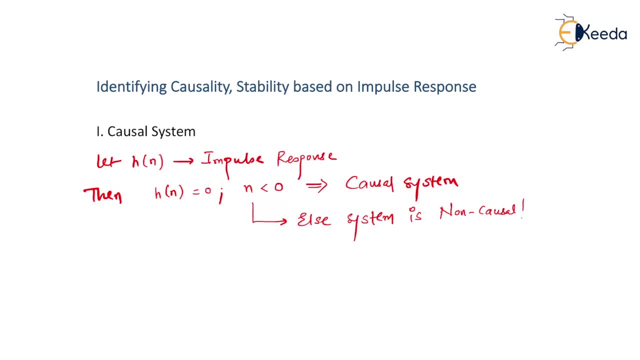 output depends on the current input, then it's said to be a non-causal system, and we know that non-causal systems are not practically realizable. in fact, all practical systems are said to be a causal system, because we cannot have a system where output depends on future input. am i right? so when a relation between output and input 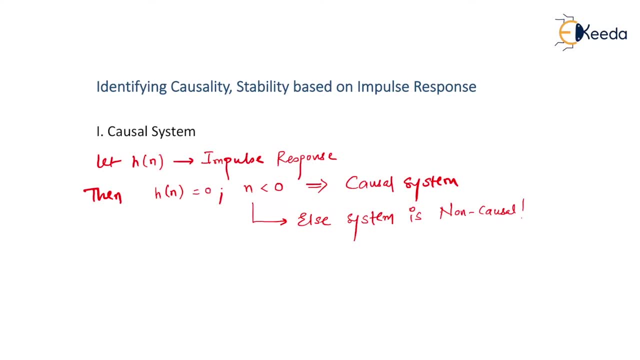 is given to you, you were in a position to identify whether the system is causal or non-causal. but this time a scenario is quite a different. this time, relation between output and input is not given to you. what is given to you is an impulse response of the system, and then you have to. 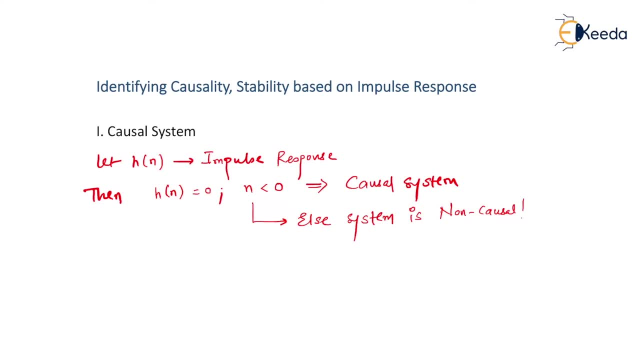 identify whether the system is causal or non-causal, and for that i have written one criteria: that h of n must be equal to zero. for n less than zero, the system is causal, and if this condition is not satisfied it is said to be non-causal. but let us understand, and let me prove it, why it is so. 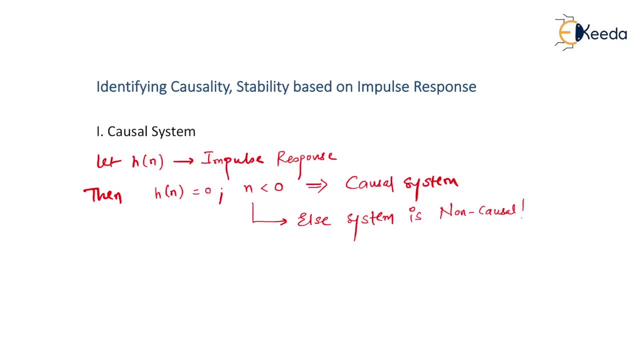 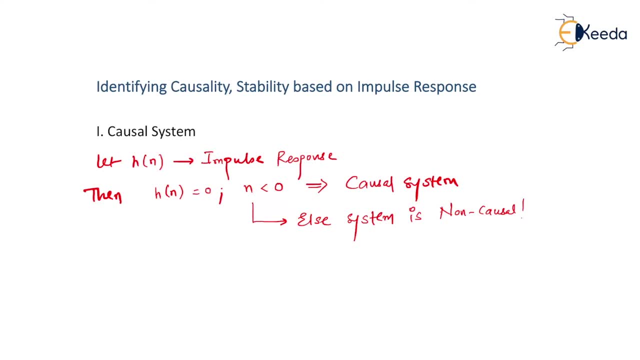 for n less than zero, how it becomes causal, otherwise it is non-causal. so first of all, we know what is the relation between x of n, y of n and h of n, that is, y of n is output, x of n is input and h of n is an impulse response. so we know that, mathematically, 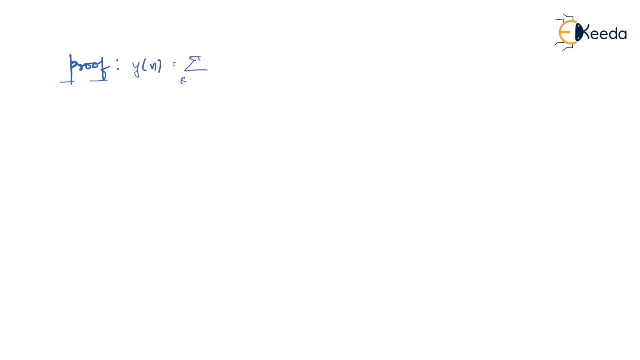 y of n is summation, k equal to minus, infinity to infinity. x of k, h of n is input and h of n is input, and h of n is input and h of n is input. so this is the relation between y of n and x of n. 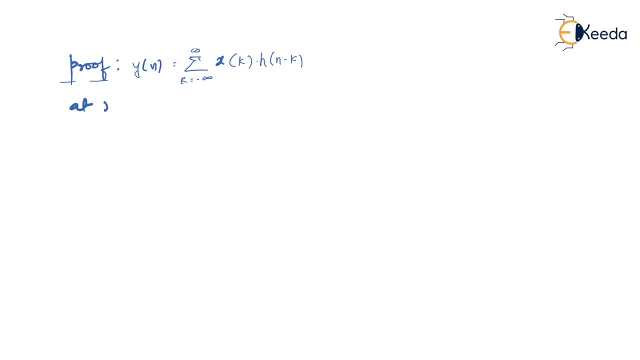 so let us assume: at n equal to zero, at n equal to zero, the above relation will become y of zero equal to summation, k equal to minus, infinity to infinity, x of k, h of minus k. am i right? so now, if i expand this summation, this y of zero will become the n minus k and h of k will become k equal to. 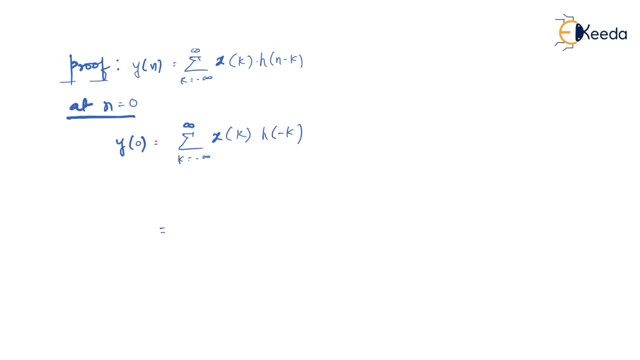 0 will become equal to okay. so we are going to vary k from minus infinity to infinity. okay. again, it is not possible, so we will expand it for some certain values of k. let us assume k equal to 0. so if k equal to 0, x of k will become x of 0 and h of minus k will also become h of 0. 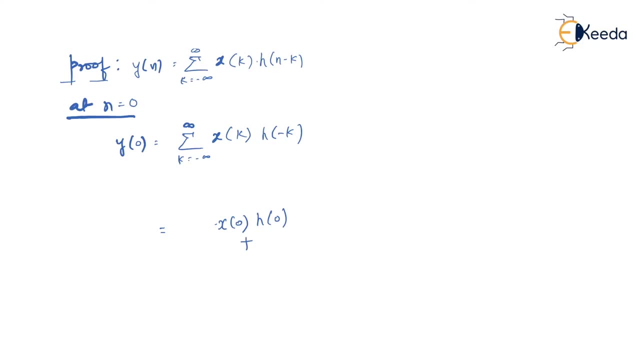 plus. now i'll go on expanding the positive values of k. so right now i have substituted k equal to 0. now let me substitute k equal to 1. so when you substitute k equal to 1, x of k will become x of 1 and h of minus k will become h of minus 1. plus let us assume k equal to 2. now. 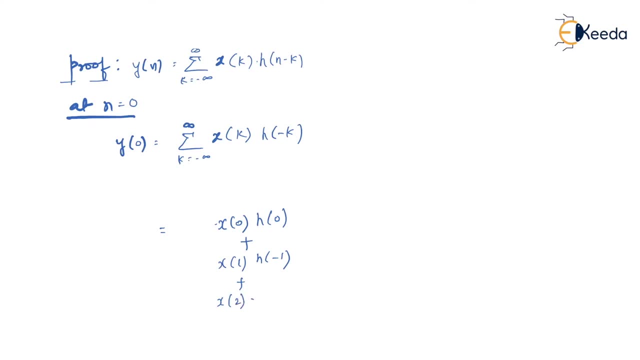 so it is x of 2, dot h of minus 2, and this will keep on increasing positively. but then k should start from minus infinity and it should go towards plus infinity. okay, so, as i said, i'll substitute certain values of k, so certain values of k, as negative, certain values. 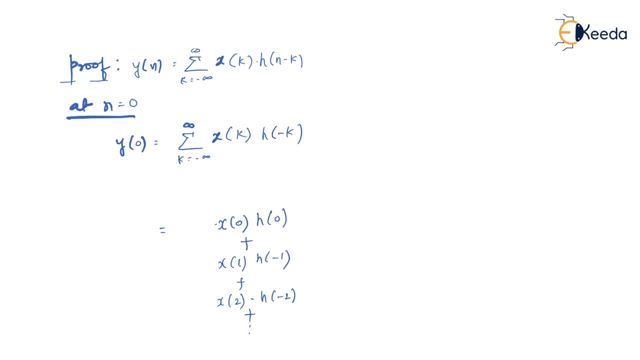 of k as positive and, of course, k equal to 0 also. i have already substituted, so only what is remaining is negative values of k. so let us substitute k equal to minus 1. so when you substitute k equal to minus 1, it becomes x of minus 1, h of minus 1 plus. 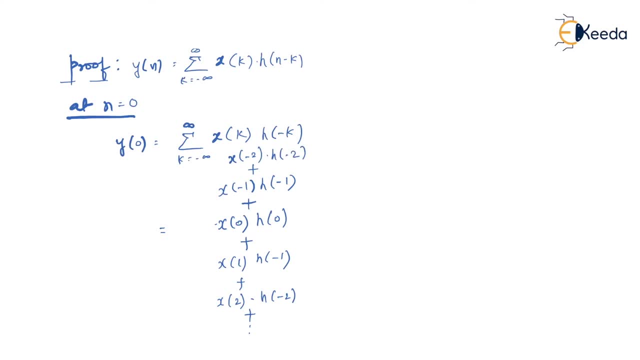 x of minus 1, 2, h of minus 2 and so on. am i right? so this whole is equal to what y of 0? please don't forget your aim. you have to identify causality of the system and i'm sure you remember when output is expressed. 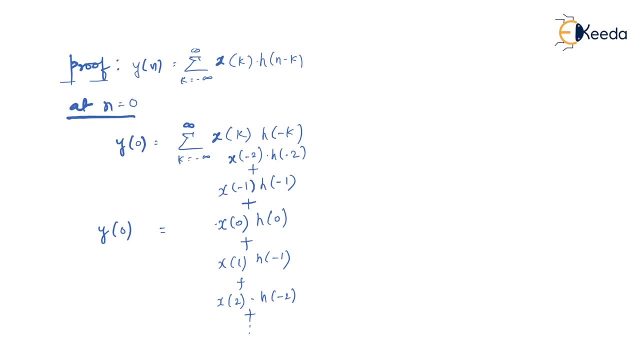 in terms of input, how to identify the causality? so this is what i have done over here. i have tried to express your output y of n, in terms of x of n. here am i right? so based on that, let's say, if you want to identify causality of the system, we know that, according to causal system, present output. 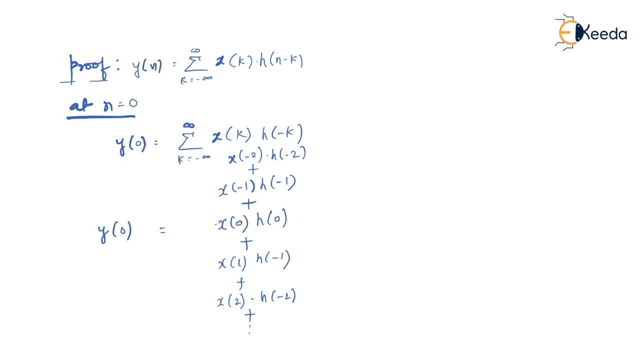 must depend on present input or at the most past inputs. but output shouldn't, you know, depend on future inputs. that is strictly not allowed for causal system. so here i can say that y of 0 can depend on x of 0, because y of 0 means it is y of n at n equal to 0, and x of n at n equal to 0 means 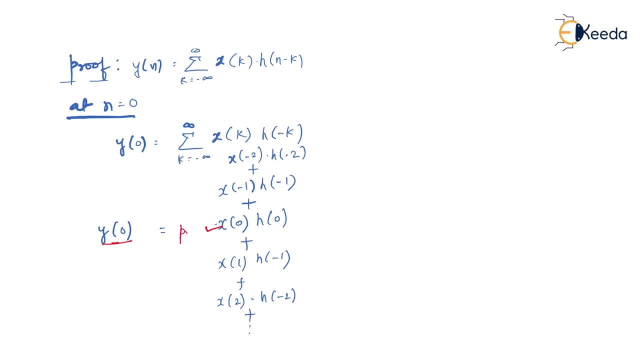 it is x of 0 and x of 0 means it is y of n at n equal to 0, and x of 0 means it is x of 0- zero. so X of zero can be treated as what a present input. so you know this is. 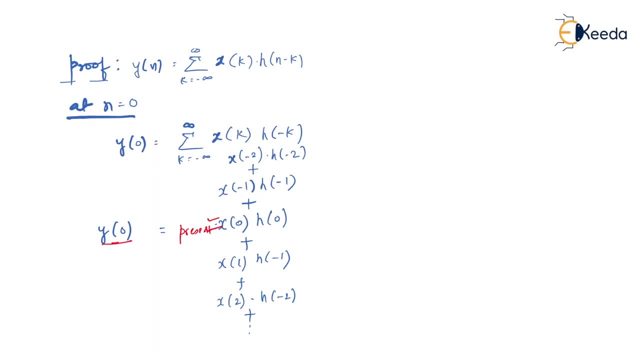 allowed. X of minus win is also allowed, because Y of zero if depends on X of minus one, it means the current output depends on a past input. so X of minus one is allowed, X of minus two is allowed, but you know what is not allowed? that Y. 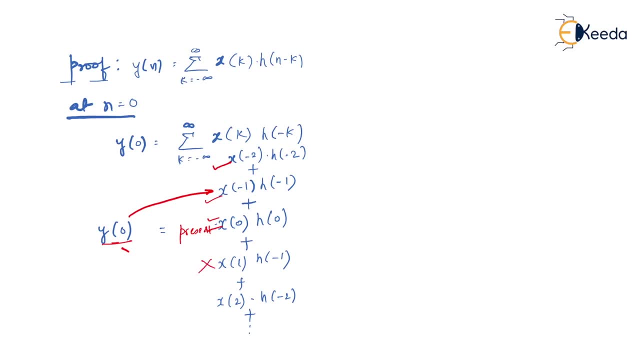 of zero shouldn't be a function of X of one, because if Y of zero- that is a present state- is taken at n equal to zero, Y of zero shouldn't depend on X of one, because X of one has become what future input? in fact, X of two is also a future input. it means it shouldn't be function of X. 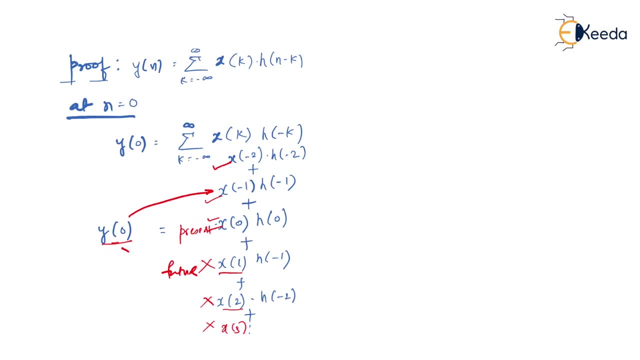 of one, X of two or X of three and so on. am i right? what does that mean? it means that this whole part should be equal to zero, and it is possible only when H of minus one equal to zero, H of minus two equal to zero. further, 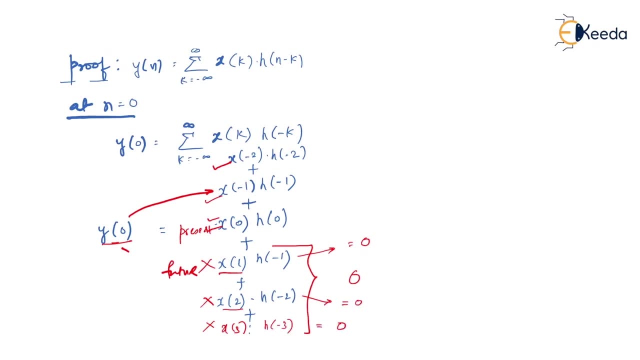 H of minus three should be equal to zero, but at the same time, H of zero is non zero, H of minus one can be non zero, H of minus two can be non zero, and so on. am I right? in fact, I should correct this to H of plus two, H of plus one, am i right? 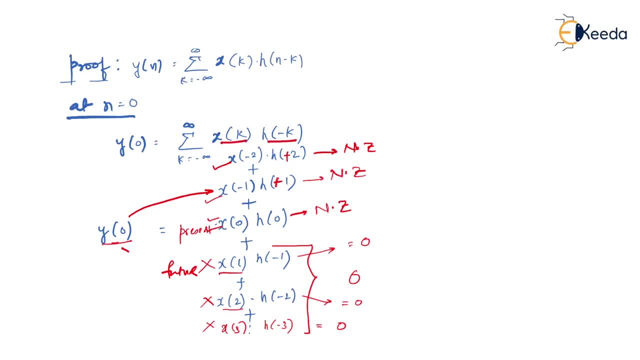 because when it is X of K, it is H of minus K. so X of minus two will accompanied with H of two, X of minus one will get accompanied with H of one, and X of one accompanied with H of minus one, and so on. so what do we see over here? 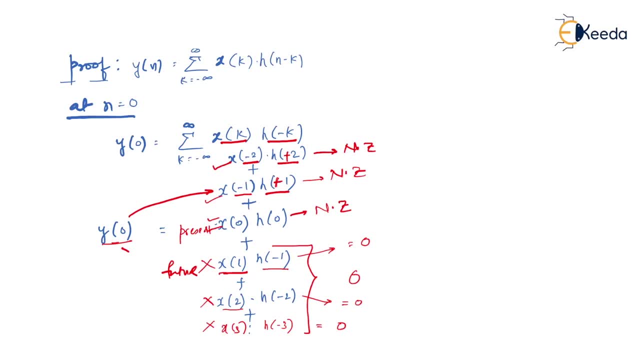 that H of n is always equal to zero when there are negative values. okay, when there are negative values, it is always equal to zero, and whenever there are positive values that there are chances that it should become non zero. so here we conclude that H of n must be equal to zero whenever n is less than zero, and 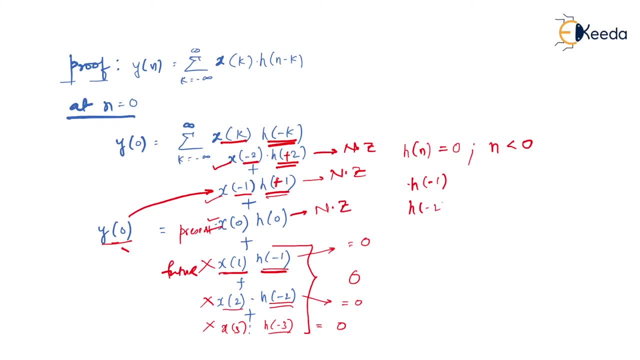 that's the reason why H of minus one, H of minus two, H of minus three should be equal to zero, am I right? so all negative values of n for H of n resulting into zero? only then the system is said to be a causal system. so please remember that. 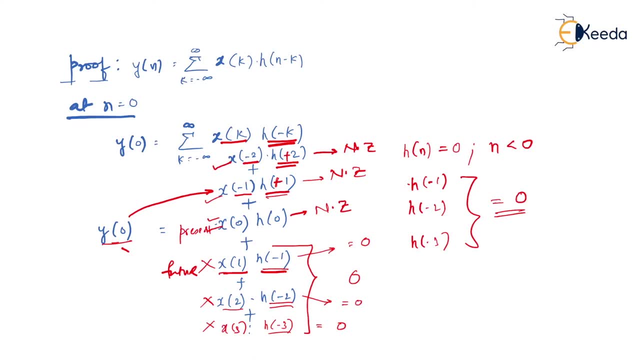 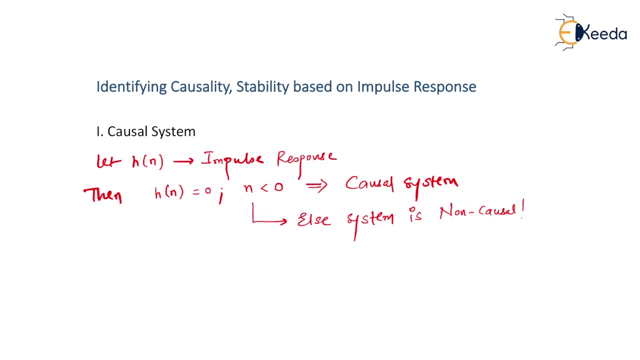 a system is said to be causal, if you want to identify it from the given impulse response, then impulse response must be zero for n less than zero, am I right? so this was the proof for causal system. please remember: whatever we have stated, it is for discrete time system, so right now it is valid for a discrete time. 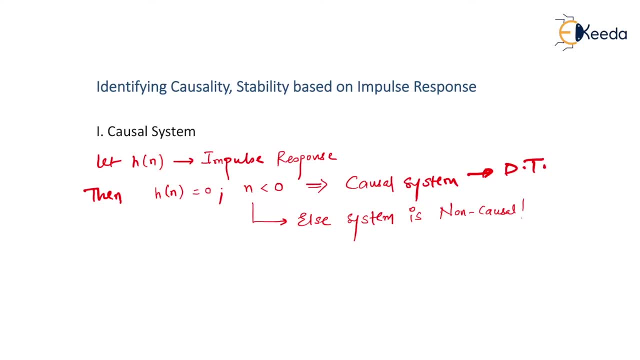 system. we can write the similar statement for continuous time system also. so we know that for a continuous time system, instead of H of n we call that impulse response as H of T. so I can write a similar statement that H of T must be equal to zero for e less than zero. 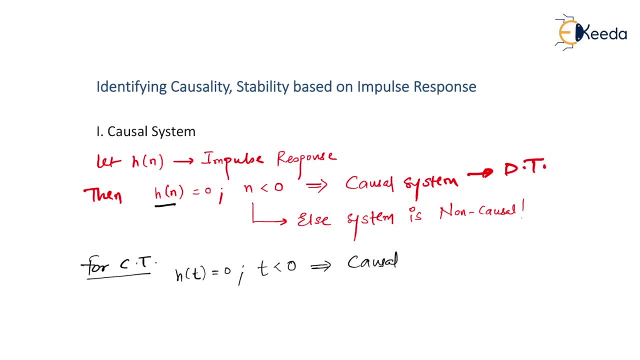 only then a system is said to be a causal system, and if the condition is not satisfied, so else it is non-causal. further, we will see how stable system is identified from the given impulse response H of n. so I'll just write the statement first and I'll prove it. 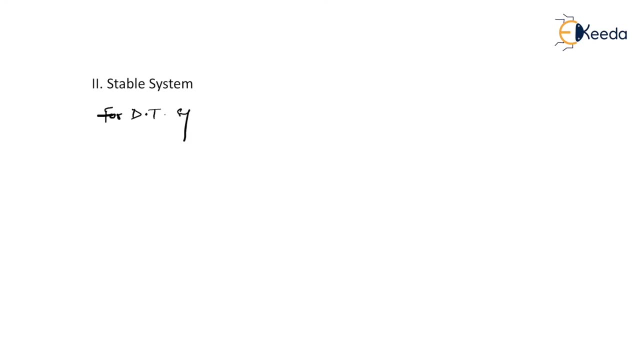 so for discrete time system we can derive the � chaparral what do we get when you get the Mia하는 method it's now the formula for any a sum of two whole SUBDI Tang mAuough of H of N when taken a summation and n is changed from"-infinity to plus infinity this must be less than infinity so I'll tell you mathematically what does that mean is H of n should be finite value I mean summation of H of n shouldn't be equal to infinite so mathematically we say that H of n must be sufficient values that localize those of H for n so this becomes evident. 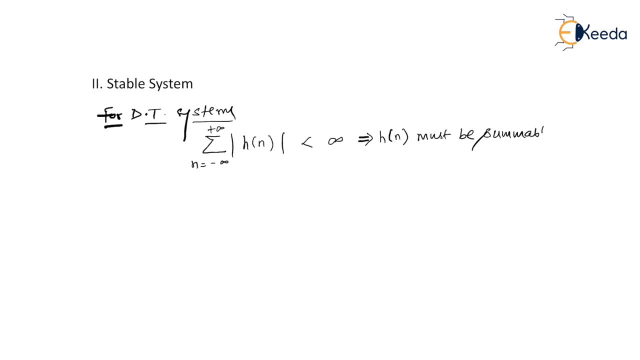 That is, after summing all the samples present in H, write from minus infinity to plus infinity. So it means all the samples present in H. if we add up them then it should result into finite value. In that case in mathematics we say that the given H is a summable one. 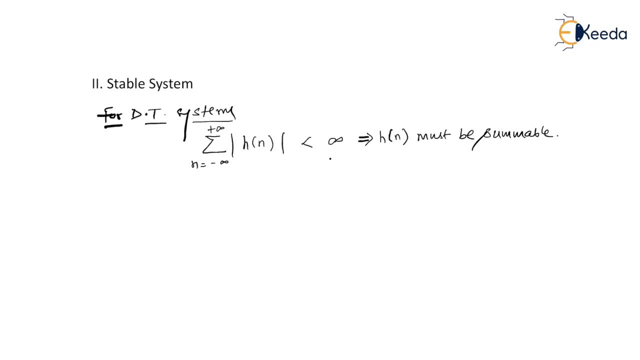 So if H is summable, then the system is stable system. So let me tell you: if it results into infinity, that is, summation n is changed from minus infinity to infinity mod of H. if results into infinity, then system is unstable. 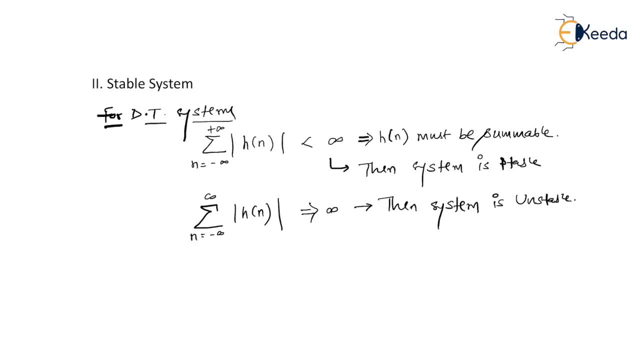 So it is in case of discrete time system, In case of continuous time system. you know that if we perform summation in discrete time system, If we perform in continuous time system, of course it is an integration and again it is vice versa, true? 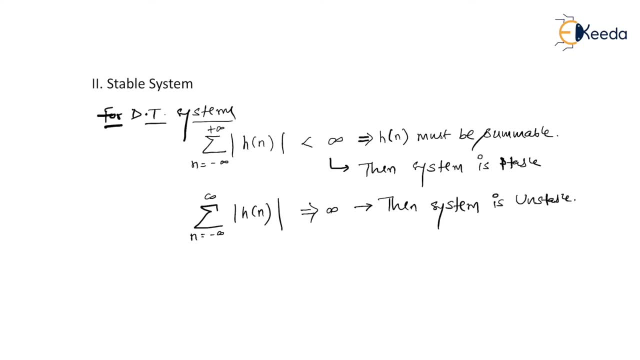 Integration in continuous time system becomes summation in discrete time system. differentiation in continuous time system becomes difference equation in case of discrete system. So in case of a continuous time system, I can rewrite the same statement as integrating over minus infinity to infinity H, d, and mod of it should be less than infinity. 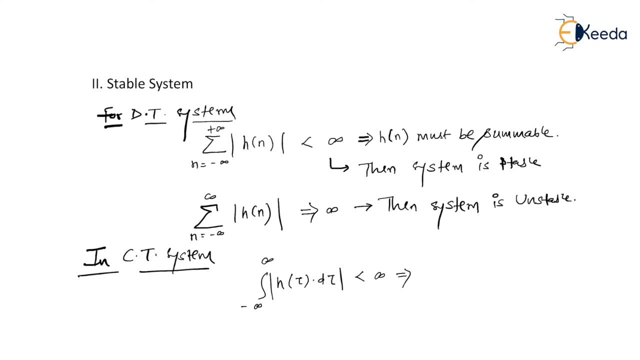 So in mathematics we say that H must be integrable. So here we say that H must be integrable or area under the curve of H should be finite. Only then the system is stable. And of course, if this condition is not satisfied, then the system is unstable. 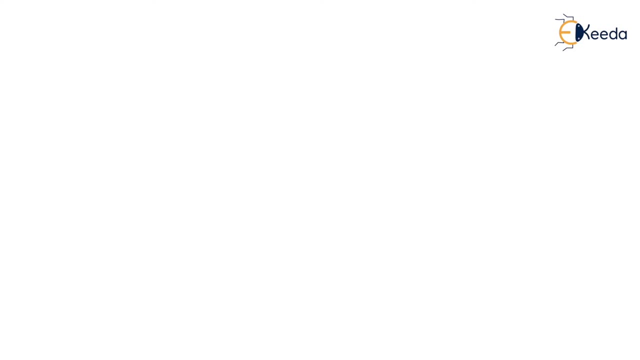 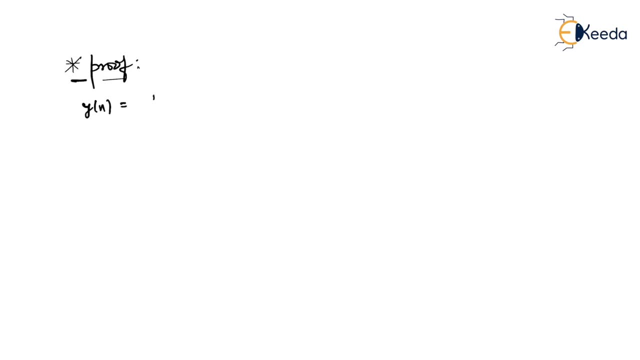 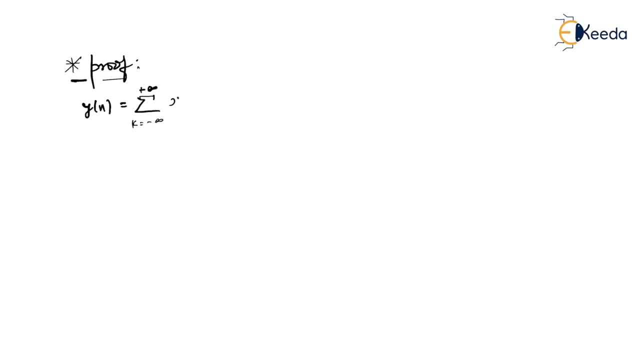 K is sumed from minus infinity to plus infinity, H and minus K. so we know that stability of the system is based on the Bebo principle, that is, Bounded Input, Bounded Output. What does that mean If the input of the system is bounded in nature, and after applying to the system, when system 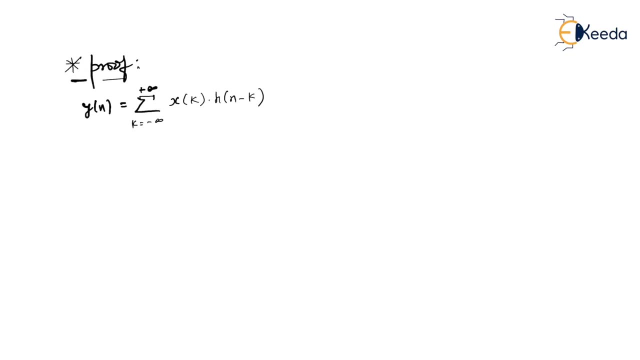 processes it and produces its own output- This is called the Bebo principle- then the produced output must also be finite. what does that mean? if finite input every time produces finite output, then we say that it is a bounded input, bounded output system. and then we say that a system is said to be a stable 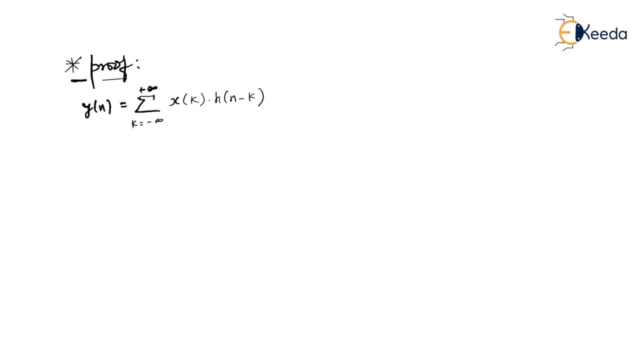 system. but if a bounded input results in unbounded output, then 100% system is unstable, is it right? so it means input is bounded, produces output bounded in nature, then the system is stable. so we know that input must be bounded first of all. so we know that for 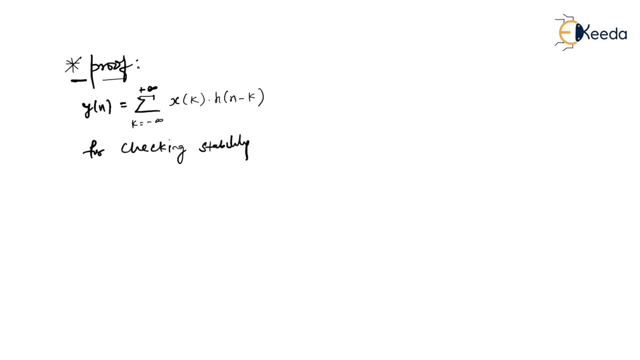 checking stability. X of K, that is, input, must be what bounded at every interval of time. X of K should be finite. so, for simplicity, what I'll do is let us assume that X of K is always 1, because 1 is what 1 is: unity. and if it, 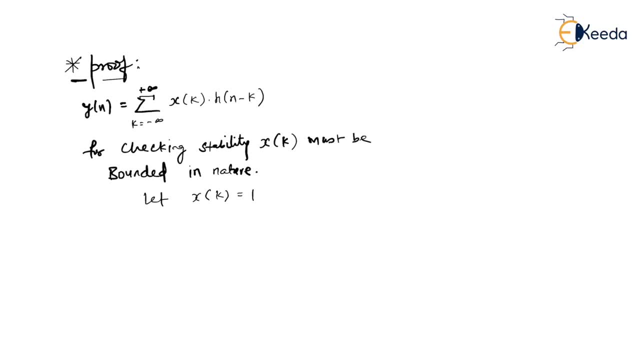 is a unity, then it can be taken as a bounded one. so let us assume X of K is equal to 1, then let us substitute this in equation 1. so I'll call this as equation 1 and I'll substitute this in equation 1. therefore, Y of n will become equal to summation where K is changed. 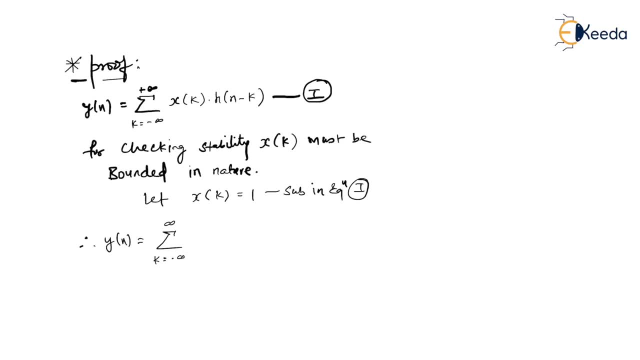 from minus infinity to infinity. X of K is equal to 1. so we did not to mention X of K. now I'll just write H of n minus K. we know that whenever a system is stable, we check a b-boe principle, that is, bounded input, bounded output. so we 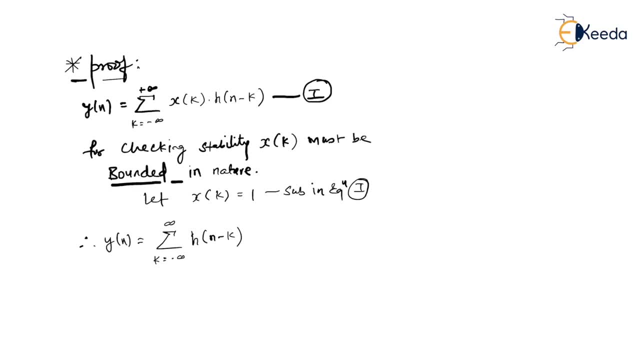 know that X of K is equal to 1, so X of K is already bounded in nature. what we have to check whether Y of n is bounded or not. so for stable system Y of n must be bounded. bounded means what it shouldn't become infinity anywhere. but then can I say: 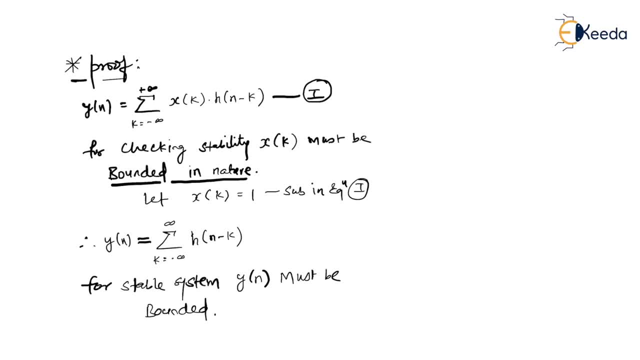 that Y of n is equal to this. summation K is changed from minus infinity to infinity H of n minus K. so if you want Y of n must be bounded, then can I say that this must be also bounded. therefore, for stability I would say that summation K equal to minus infinity to plus infinity H of n. 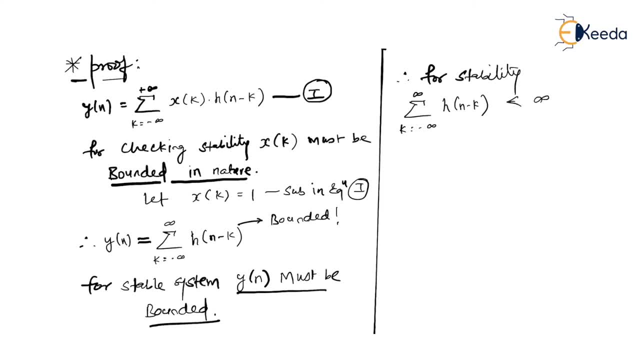 minus K should be less than infinity. am I right? let me tell you, this whole will become less than infinity. ok, only when the original term H of n should be also less than infinity, because, understand, H of n minus K is derived from H of n. let me be very clear about it. 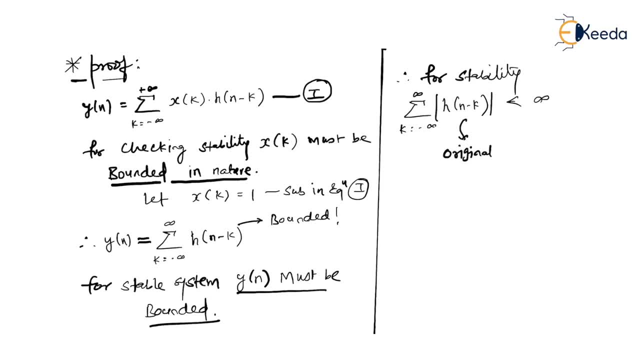 this is originated from H of n, am I right? then we must say that an equal to minus, infinity to infinity, mod of H of n should be as well as than infinity. so now we are coming back to this story that if you want a system to be stable, then mod of H of n where n is. 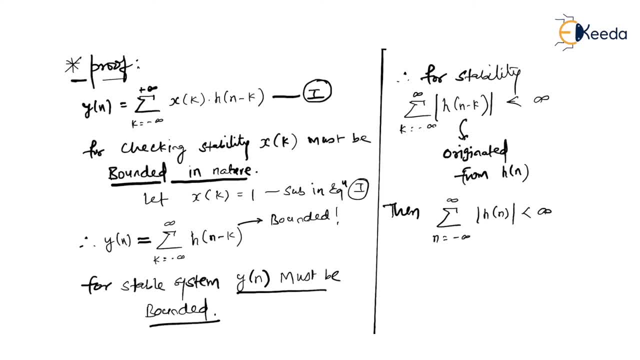 change from minus infinity to infinity should result into a finite value. what does that mean? that if the H of n is given to you and if you add all the same inside h of n, it must be less than infinity, and only then the system is said to be a stable system. 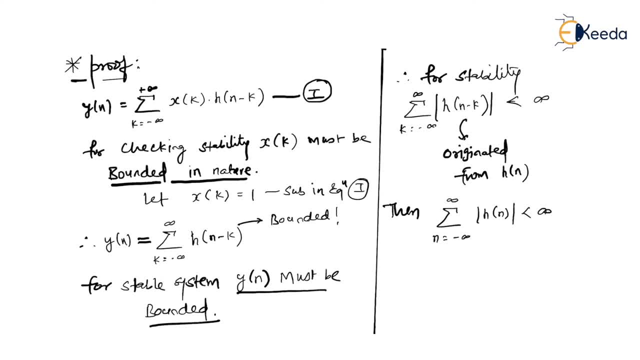 so this is how we have proved for discrete time system. similarly, for continuous time system we write this way: integrating over minus infinity to infinity. h of tau, d, tau and mod of it should be less than infinity. so this is for a continuous time system. so for continuous time system, h of t. 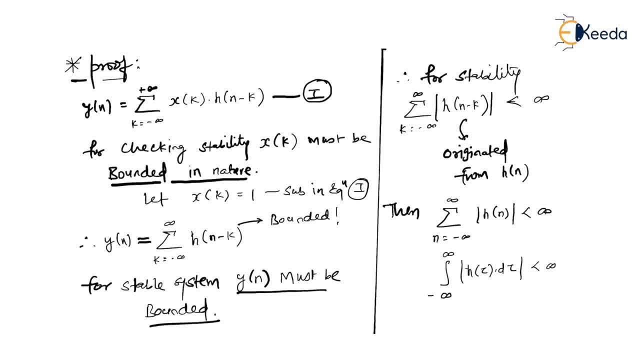 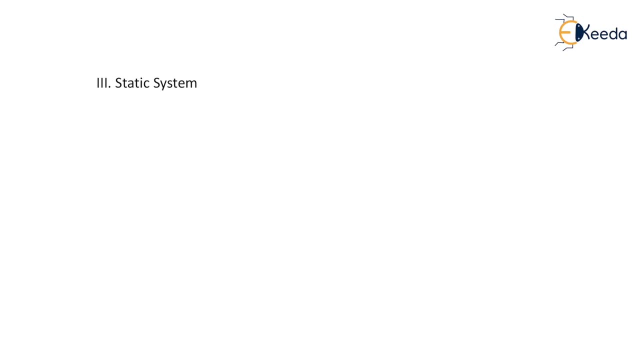 must be integrable and for discrete time, system h of n must be summable. only then the respective system is said to be a stable system, whether it is discrete or continuous time. now the last thing. we will see how to identify whether the system is static or dynamic, depending upon the given 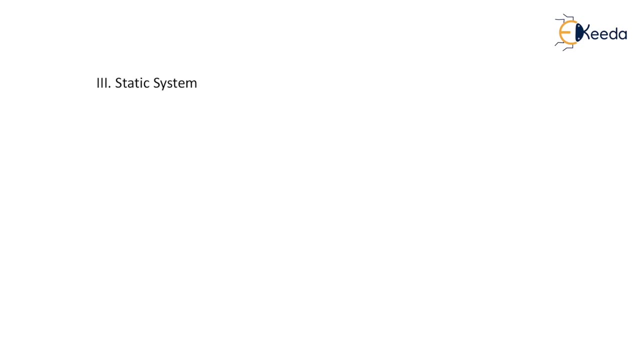 impulse response because we know that we already have studied this- how to identify a static system or dynamic system- if the relation between output and input is given to you. so let me remind you that we have already studied this: how to identify a static system or dynamic system. 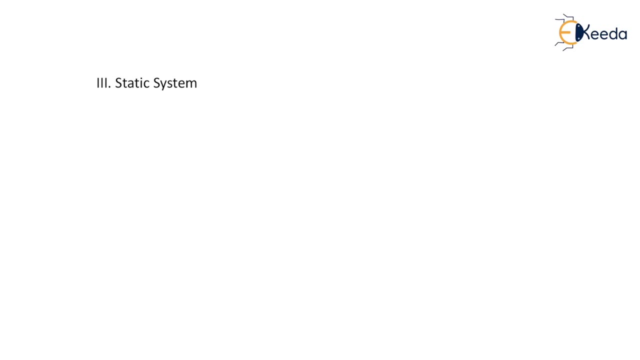 for static system, output or current output must depend on present input. only that is present. output should be function of present input. only that is present. output should not depend on future input or past input, am i right? so let me remind you: for static system, present out must be a function. 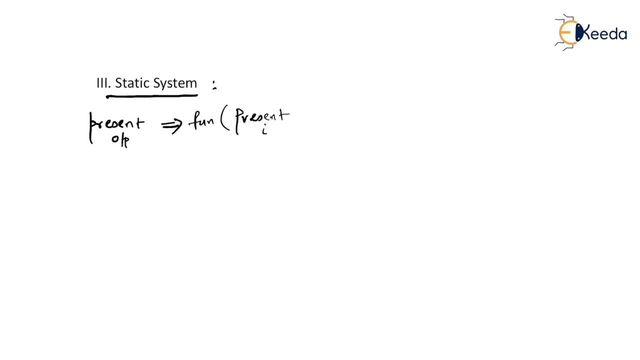 of present input. only only then the system is said to be a static system. so from impulse response point of view, we write it this way: h of n should be equal to zero. when n is not equal to zero, then the system is said to be a stable system. okay, let me correct it. we should write a static system, am i right? else system is: 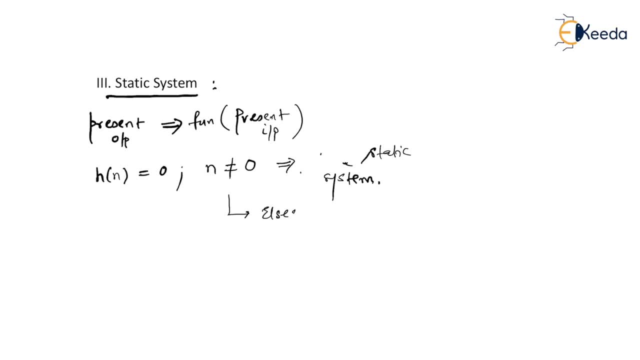 said to be a dynamic system. so now we need to prove this. why h of n should be equal to zero. when n is not equal to zero, then only it is a static system, else it is a dynamic system. so let me prove it from the similar relation. 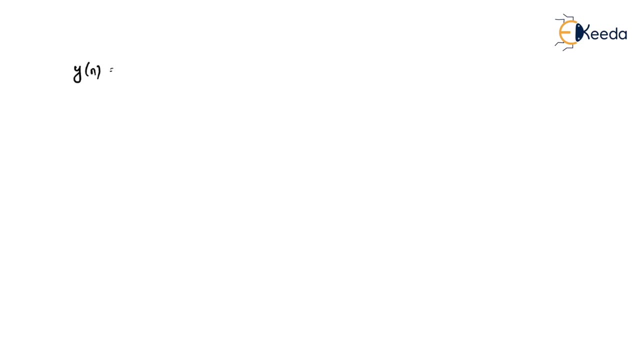 i'll do that. let us assume y of n equal to k, equal to minus infinity to infinity, x of k, h of n minus k. so of course it is not under any assumption. this is a true relation between y of n, x of n and h of n, with the help of a convolution summation. 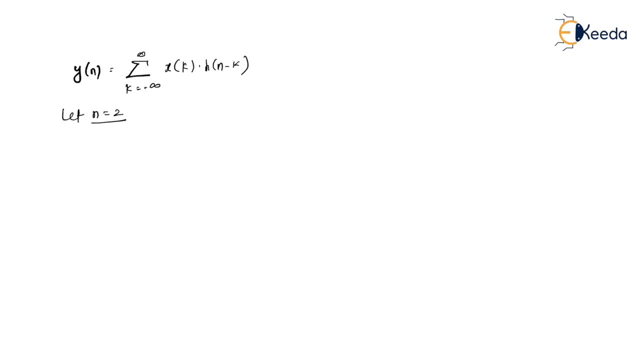 so let me substitute n equal to 2, then can i say: this is equal to y of 2, which is equal to summation, k equal to minus infinity, to infinity x of k, h of 2 minus k. am i right? so now expand this by substituting: 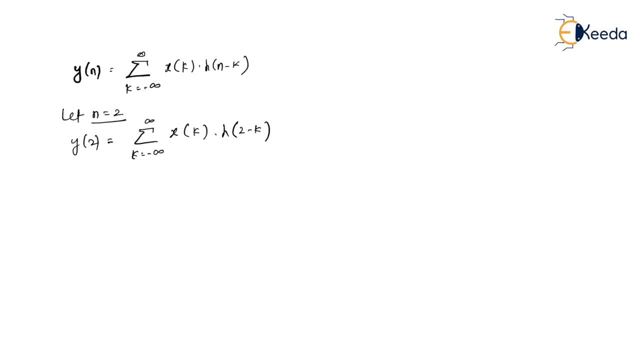 certain values of negative values of k, also k equal to 0 and certain values of k which are positive values. so now this is y of 2 relation. let me substitute k equal to 0 first. in that case it becomes x of 0 dot, h of 2 itself, plus now i'll go on expanding all positive values of k. 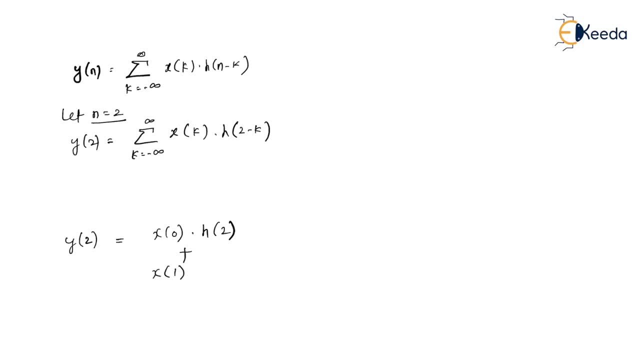 in that case it will become x of 1, that is, at k equal to 1, dot h of 1 plus x of 2, h of 2 plus x of 3. in fact, this will become 0. am i right? because whenever you substitute k equal to 2, so it is. 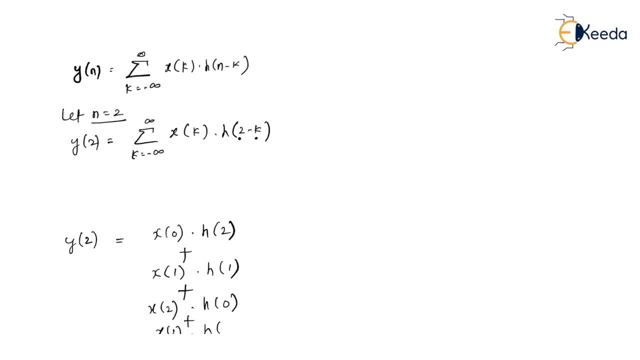 2 minus 2, it is 0. then let us substitute k equal to 3: 2 minus 3 it is minus 1, and so on. am i right? so let us substitute negative values of k now, so it becomes x of minus 1. so when k value equal to minus 1, 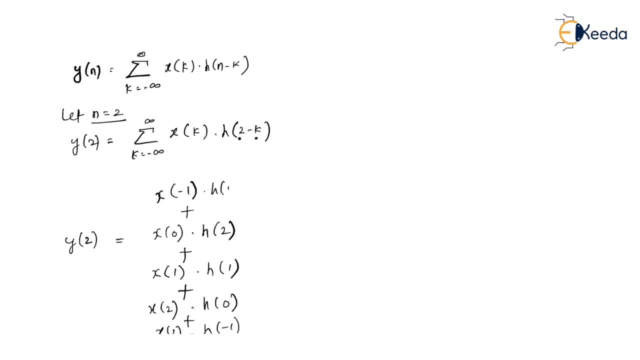 2 minus of minus 1 will become h of 3, and so on. am i right? so now this is a y of 2 relation with respect to x of n. now concentrate on the negative values of k now. so let us substitute negative values of k now. 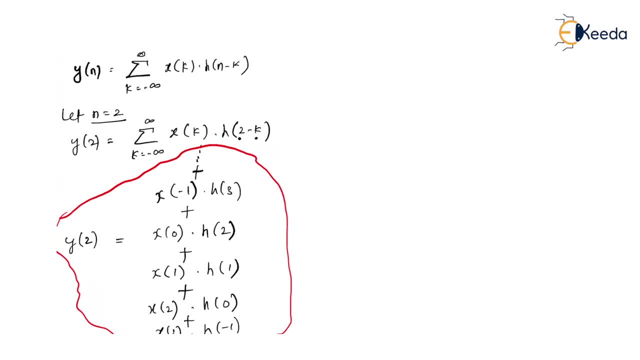 on the thing that we need to really prove. we need to prove whether the system is static or not. okay, so for static system, we know that, that the present output must depend on present input only. so if i say y of 2 as present output, in that case x of 2 is called as a present input. 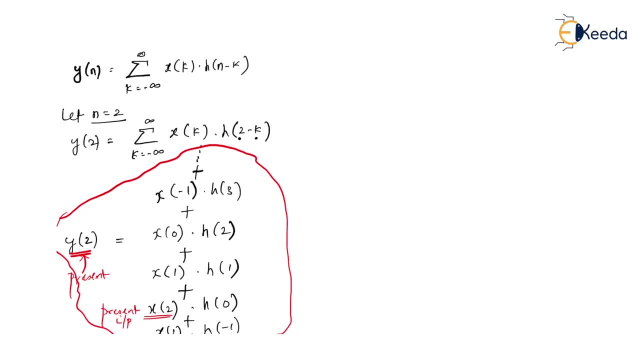 is that right? it means output and input must be seen at the same instant of the present input. so if i say y of 2 as present input, what does that mean? that y of 2 should not depend on x of 1, because x of 1 is becoming a past input. in fact, x of 0 is also a past input. 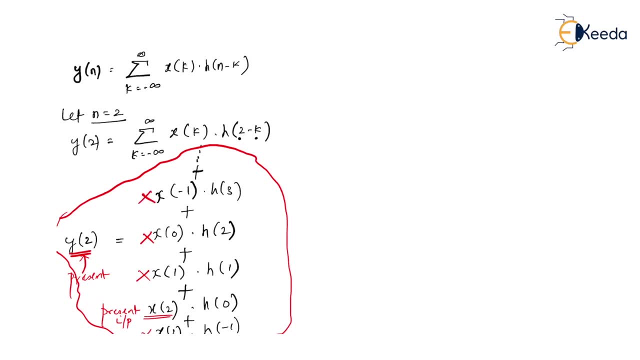 x of minus 1 is also a past input. x of 3 is nothing but a future input. so what does that mean? if you want your y of 2 should be only function of x of 2, then h of 0 must be non-zero. at the same time, if you want that y of 2, 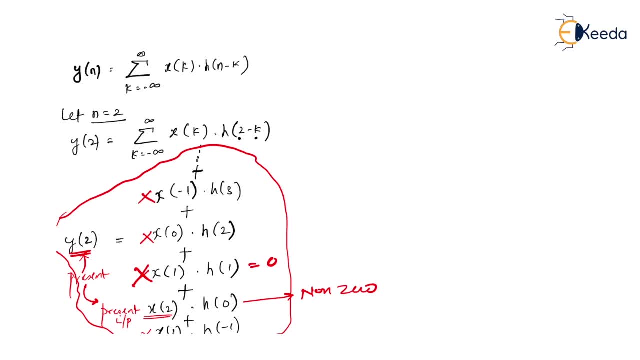 must be non-zero, then h of 0 must be non-zero. if h of 0 must not depend on x of 1, then h of 1 should be equal to 0. also, h of 2 should be equal to 0. h of 3 should be also equal to 0. 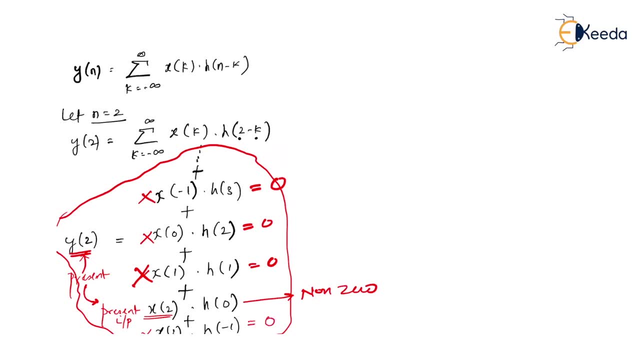 h of minus 1 should also become equal to 0. if you want y of 2 should not depend on x of 3, what does that mean? if you want your y of 2 to be depend on only on x of 2, only h of 0 should be non-zero. so here: 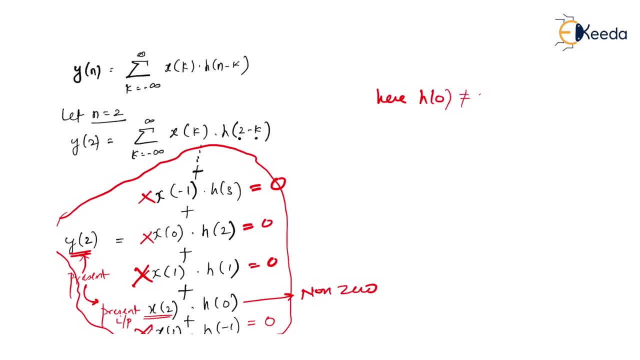 h of 0 is not equal to 0, but every time you see that h of n is always 0 when n is not equal to 0. is that right? so this proves that if you want a system to be a static system, h of n should be equal to 0 for n not equal to 0. so it means h of 0 only should be non-zero. 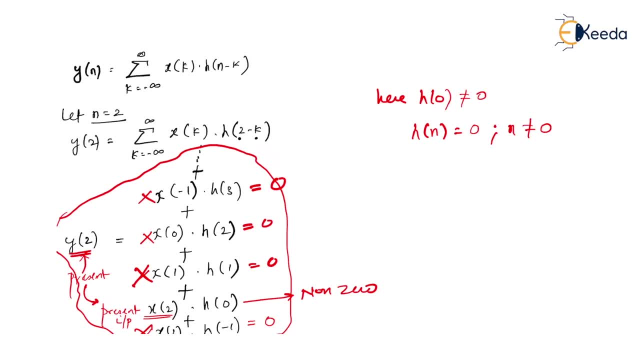 else h of 1, h of 2, h of 3 should be equal to 0, h of minus 1, h of minus 2, h of minus 3 should also become equal to 0. only then a system is said to be a static system. otherwise it is a dynamic. 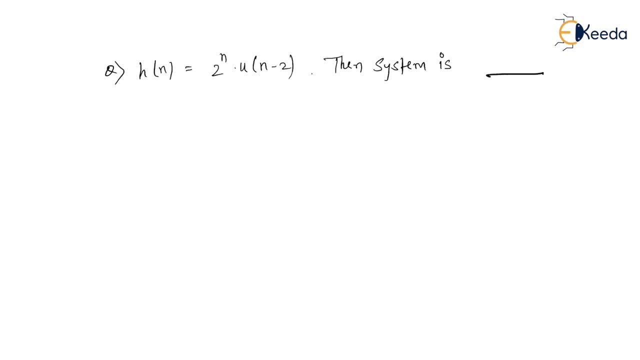 system. let us solve one problem. so i kept this problem in general. that is, some h of n is given, which is 2 raised to n, u of n minus 2, and the system is: but then deliberately i have removed all the options because i want to solve. 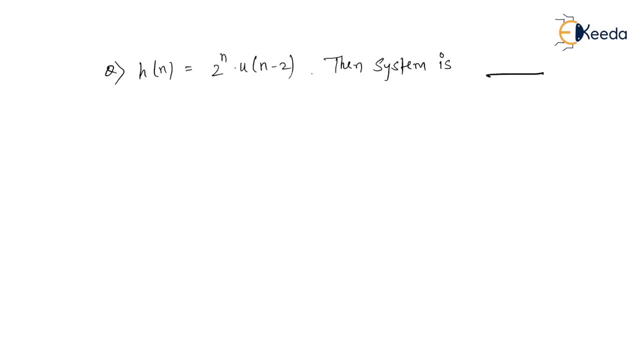 this problem for every aspect that we have learned. so we have to see whether it is causal, non-causal, we have to check whether it is static or dynamic and at the end we will also see whether it is a stable system or unstable system. let's see. so first of all, i'll check for causality. 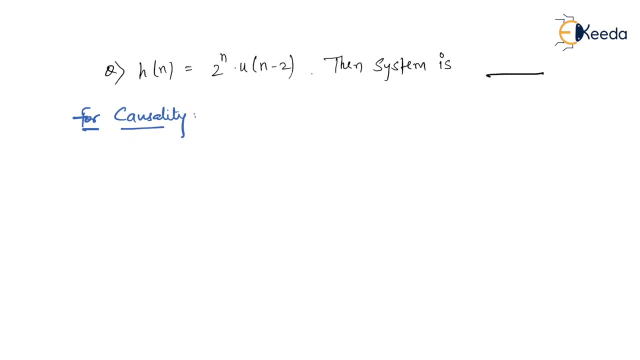 so let me remind you, for causality, h of n should be equal to 0. for n less than 0, let us give a check: h of n is equal to 2 raised to n dot u of n minus 2. so let me remind you, when i say 2 raised, 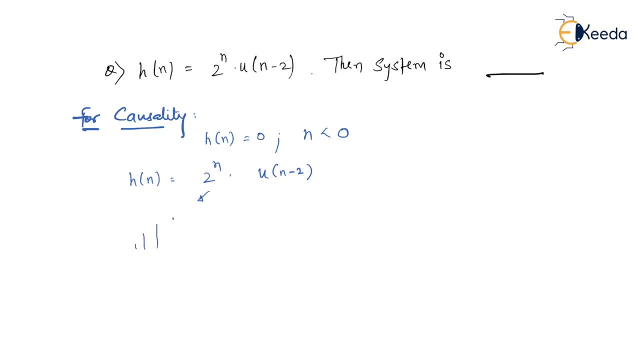 to n. it is this kind of function that is exponentially rising function, which is present from minus infinity to plus infinity, am i right? whereas u of n minus 2 is present only from 2 to infinity. so for 2 it is 1, for 3 it is 1. for n equal to 4 also, it is 1. 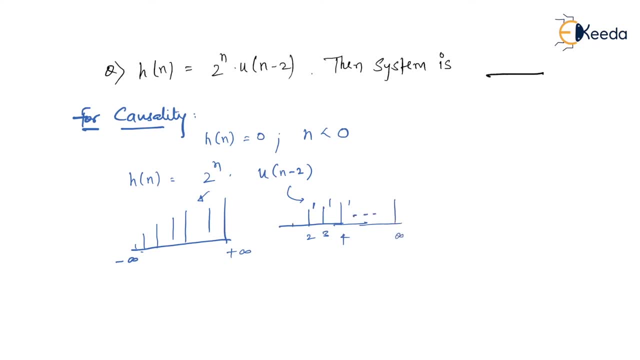 and it is going up to infinity. but then, when n is equal to 1, n equal to 0, it is always 0, am i right? so imagine if these two functions are multiplied? okay, if these two functions are multiplied, then we'll get a resultant signal from 2 only, and this will go up to infinity, am i right? 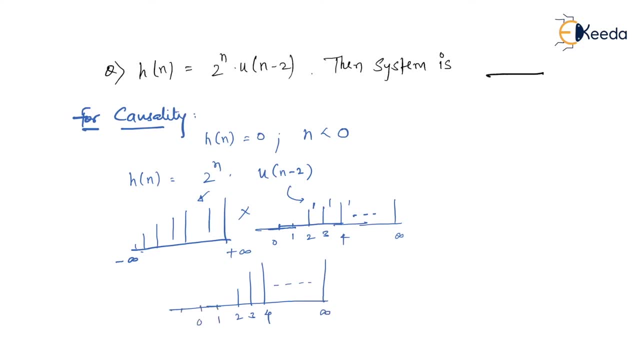 so this is 0 n equal to 1, n equal to 0, n equal to minus 1, and so on. so this is a nature of h of n. now am i right? so, if you see carefully, h of n is always 0 whenever n is less than 0. so for all. 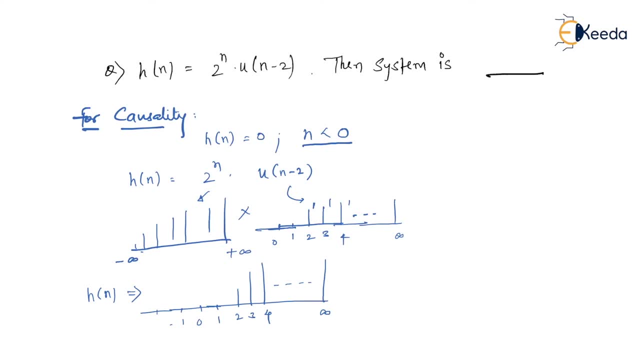 negative values of n, you observe that h of n is always 0. in that case, what i'm going to do is i'm going to say that the condition is getting satisfied and therefore a given system is a causal system. so from observation, you see that h of n is always 0 for all negative values of n. 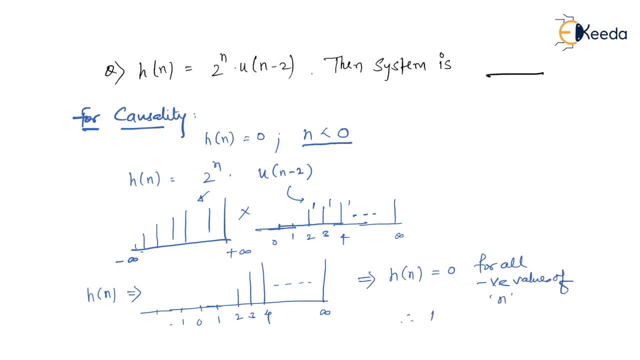 hence it is a causal system, is that right? so let us check whether the system is a static or dynamic. is that right? this is what is given to us. we know that, for a static system, h of n must be equal to 0 when n is not equal to 0, am i right? so let us check randomly. 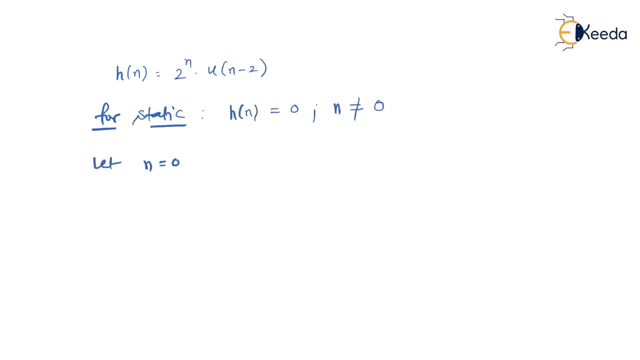 let n equal to 0, so at n equal to 0, h of 0 will become 2 to the power 0 and you have to check u of n minus 2 at n equal to 0. see, whenever you have to substitute n equal to 0, you cannot substitute blindly n equal to 0. 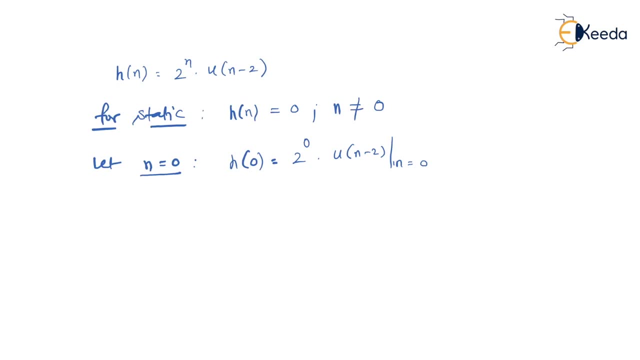 and write u of n minus 2 as u of minus 2. no, you are not allowed to do that. whenever you are substituting n equal to 0, then you have to check it this way: u of n minus 2 at n equal to 0. try to. 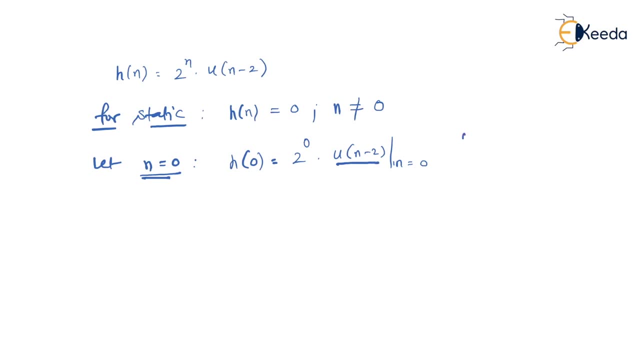 understand. u of n minus 2. u of n minus 2 function is something which is present as a step function or a unit step function present from 2 to infinity. is that right? so if you check the status of u of n minus 2 at n equal to 0, of course it is equal to. 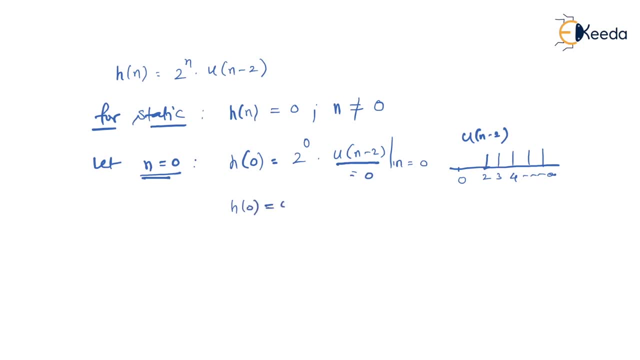 0. it means h of 0 is equal to 0. please understand. h of 0 is equal to 0. in static system, h of n should not be equal to 0 when n equal to 0. please understand this. but i'll give you one more value. okay, so i'll check. for n equal to 3, for n equal to 3, h of 3 will become. 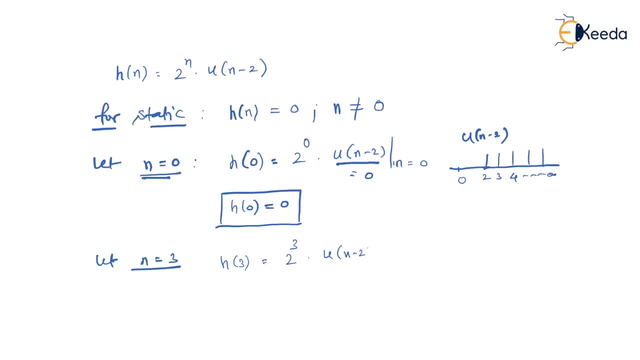 how much it is 2 to the power 3 and you have to check u of n minus 2 status at n equal to 3, is that right? so, as you can see, at n equal to 3 it is 1. so at n equal to 3 it is 1 and 2 to the. 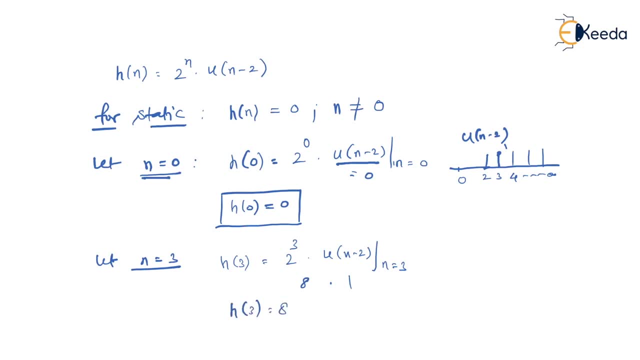 power 3 is 8. what does that mean? h of 3 is equal to 8, and let me tell you it is not equal to 0. i'm checking whether it is not equal to 0 because my condition says for static system that h of n should be always 0 when n is not equal to 0. so this is how it is not following. 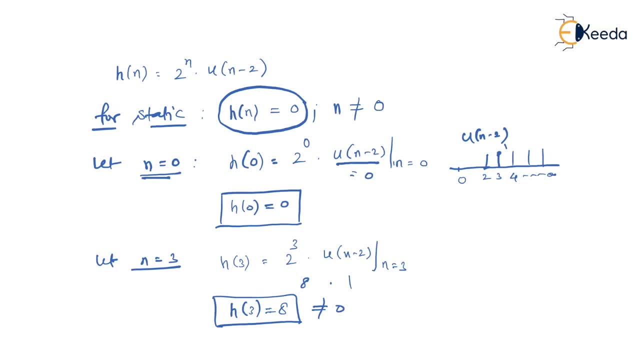 this principle and therefore the system is said to be a dynamic system. therefore, this is a dynamic system and finally, we have to check whether it is stable or unstable system. we know that, for stability, if we do summation of all samples present in h of n, if resulting into finite value, only then 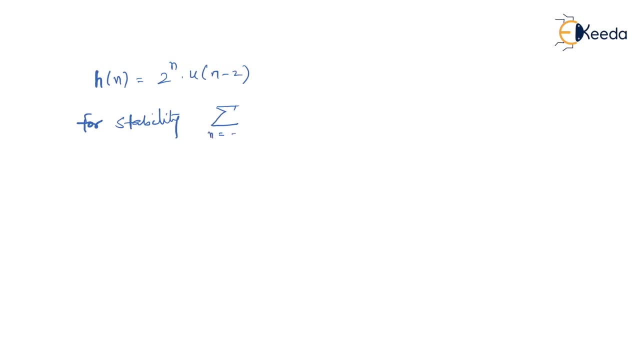 the system is said to be a stable system, that is, when n is moved from minus infinity to infinity. mod of h of n should result in finite value. is that right? so let us check, see, we know that u of n minus 2 is always equal to 1. for n greater than or equal to 2, is that right? it means u of n. 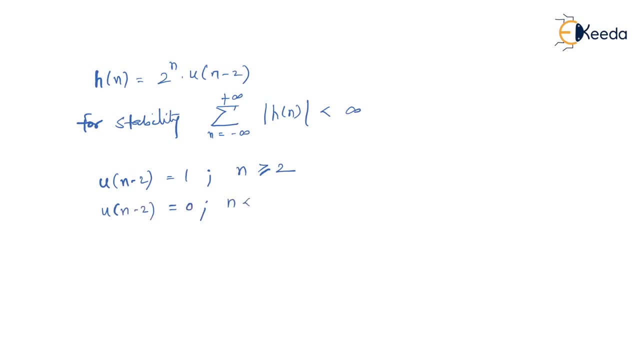 minus 2 is always equal to 0 when n is less than 2. is that right? so now i can actually make h of n as a sequence form. so here i'll write it for h of n at n equal to 0. we know that. at n equal to 0. 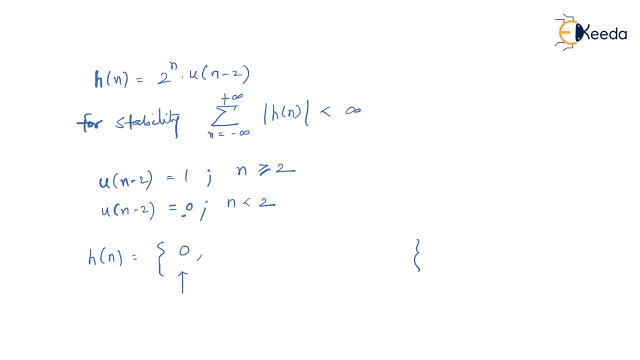 u of n minus 2 is 0, so this will result into 0. in fact, at h of 1 also, it will remain 0. at n equal to 2: okay, from n equal to 2 onwards, only this function is present. so at n equal to 2, 2 raise to 2 will become. 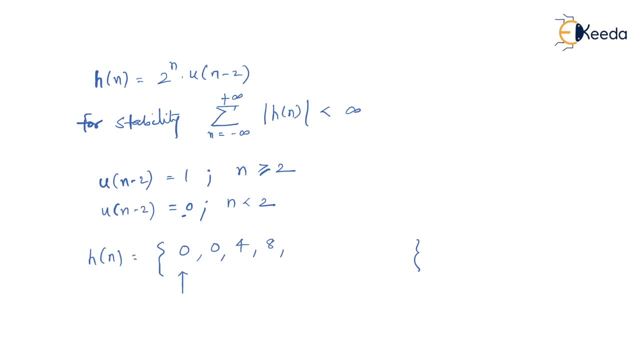 4, 2 raise to 3 will become 8, then 16, and so on. okay, so this is something which is never going to end. and if I do a summation of h of n, this is equal to okay. now, if I start summing all the samples, 0 plus 0 plus 4 plus 8 plus 16, 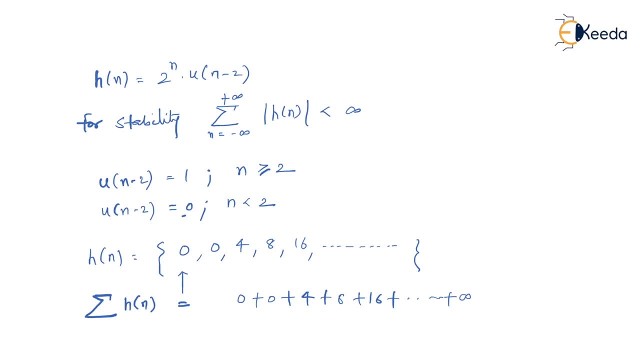 and so on. this is, in fact, going up to infinity. that is never ending, and this will result into infinity. in fact, this is is tending to infinity. in that case, I said that that this is not followed. okay, this requirement is not fulfilled and therefore the given system is. 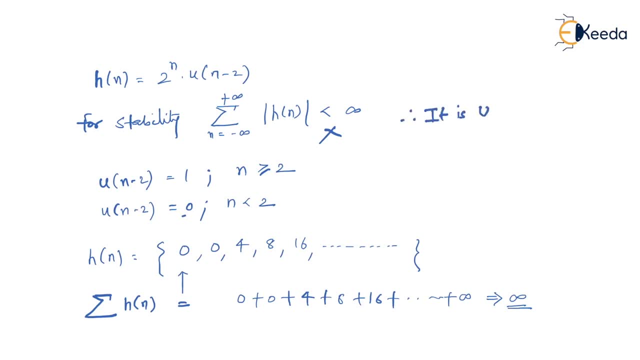 unstable system. so it is very much required that you should know how to identify the system's characteristic from the impulse response. you should be in a position to identify whether the system is causal, non-causal, whether the system is stable or unstable, or you should also understand how to identify whether the system is static or dynamic, if only impulse response is given. 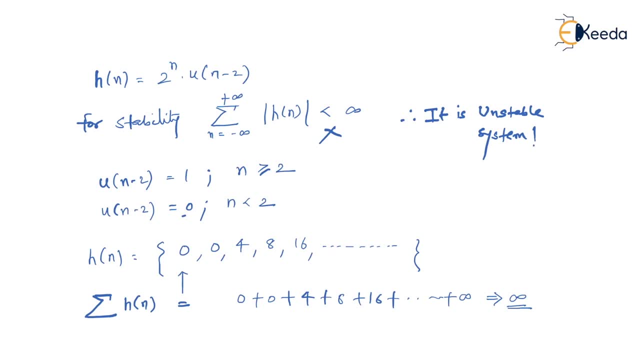 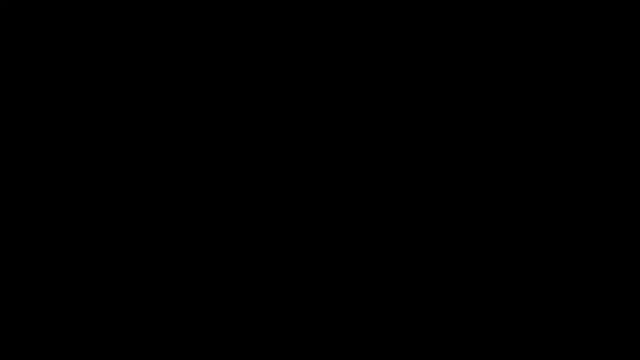 instead of establishing output and input relationship. is that right? thank you you.